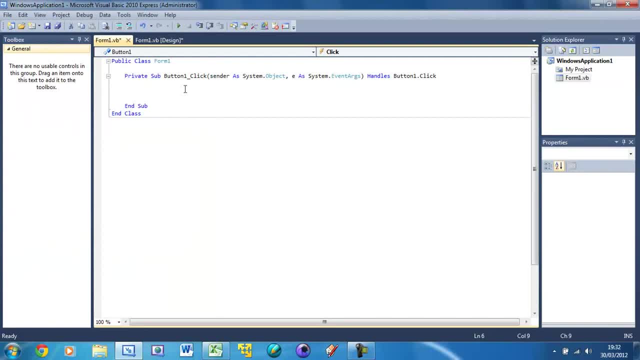 So double click on the button And you should see button one click And in here we need to declare a couple of variables. So declare total as integer, Declare first As integer And declare second As integer. So total is going to hold the total once you've added them together. 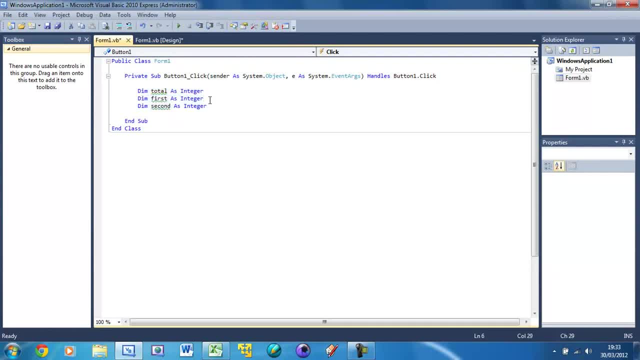 First is going to hold the first number that we're adding. Second second number that we're adding. So make some space between this And now we're going to actually declare we'll set the value for first and second. So we're going to set first. 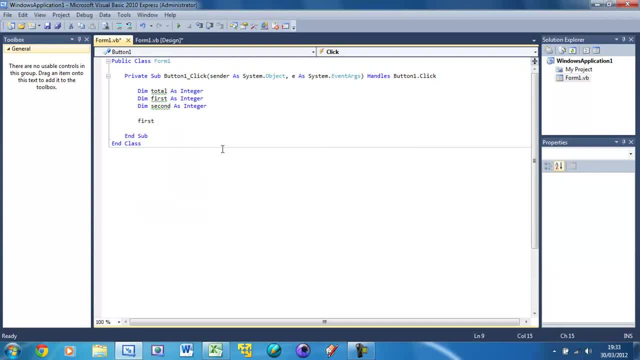 So we're going to set first equals text box, one dot text, Then the same for second equals text box, two dot text. So that's fairly simple. So make some more space. So this is declaring what they're equal to. Now we're going to actually add them up. 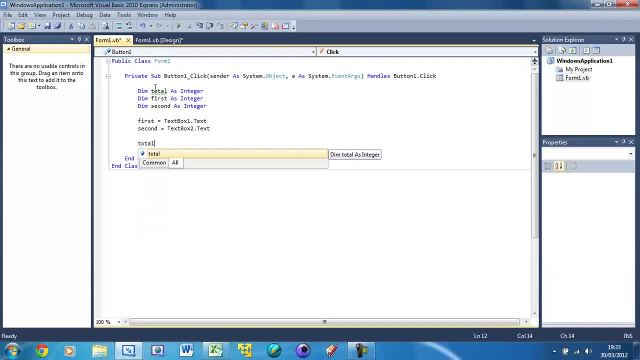 So we're going to do total. So the total variable up here Equals first plus second. That makes some more space. And now we're going to display a message box with the final answer. So we're going to do message box dot show. 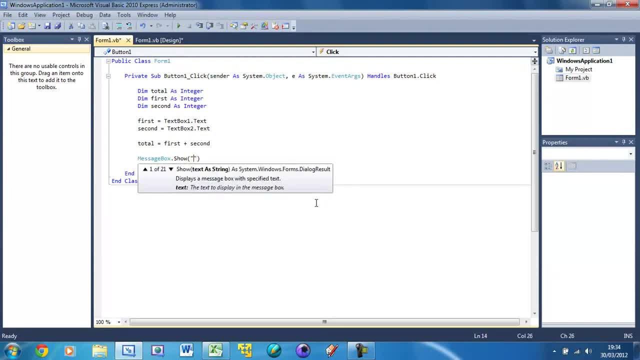 Put the brackets And in here we're going to put answer And then a colon, Then it's important that we have a space. I think I talked about this in a previous tutorial, But if I didn't. basically we put the space in to break up this word from the next word or number or whatever. 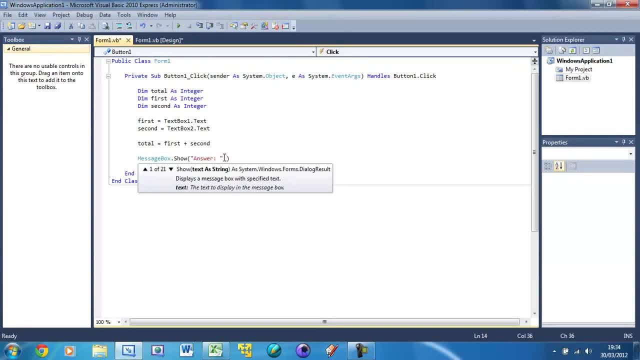 So outside of the quotations we're going to put the and sign. So shift and seven. And the reason we're putting this and not the plus is because we're dealing with numbers here And, as you can see, I used the plus here to add them together. 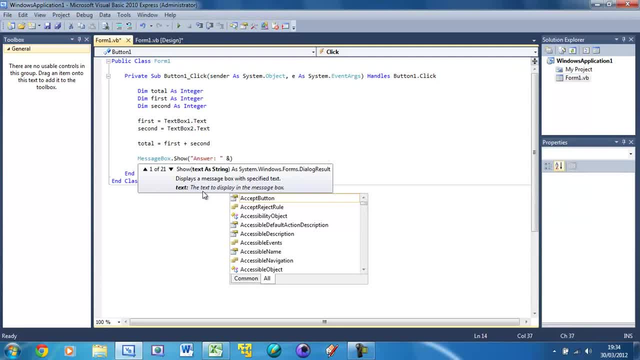 Because we're dealing with numbers, We're putting this instead of the plus. If we were to put the plus, it would attempt to add them together And since this is a number, it would fail that and it would give us an error. 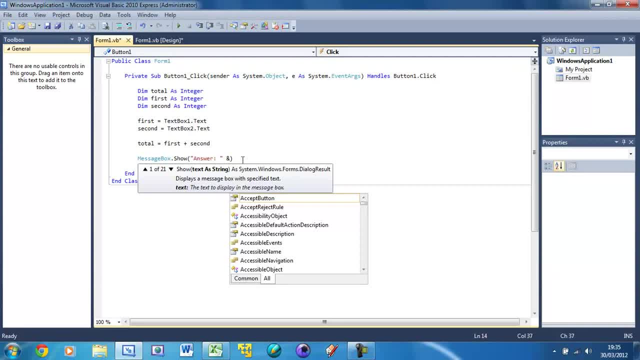 So we put this and sign here This one you can use anywhere. This is actually probably better to use, But never mind. So you put and And then total, So just like that. So it's going to show the answer: colon and then total. 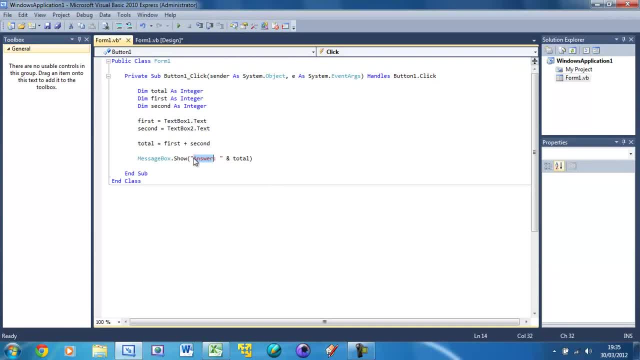 So if it's ten it's going to show answer colon and then total Answer colon, space ten. So that should be ready to run. So if you run that, no errors. So we can put two numbers. 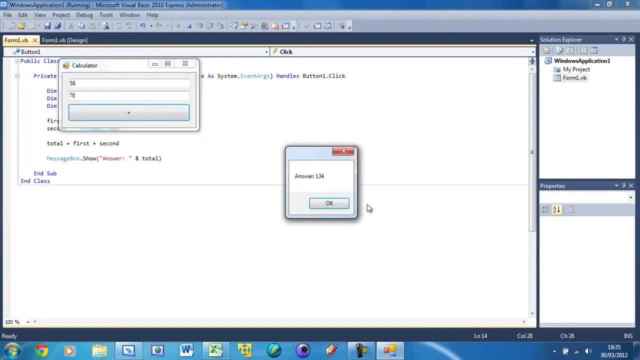 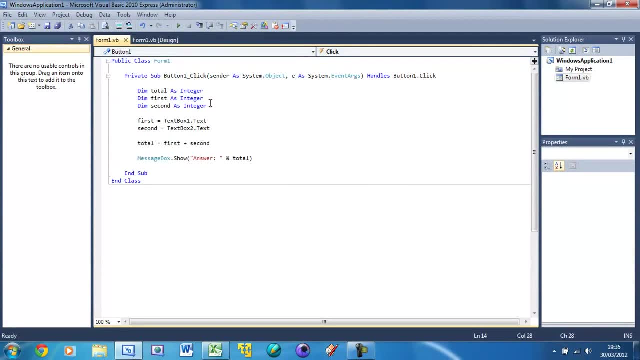 So 56 and 78. Add them together. Answer 134.. Which is correct. So if you close all of this, make sure it stops up here And I'm going to copy all of this text. As you know, I'm not going to copy that. 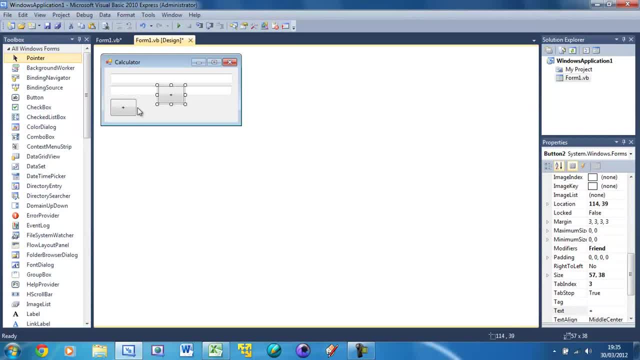 I'm going to make this smaller Copy that. Paste it three more times So that we've got four buttons. Make your form just look nice, Make it all line up. Then I'm going to change these buttons, the text of them to minus times and divide. 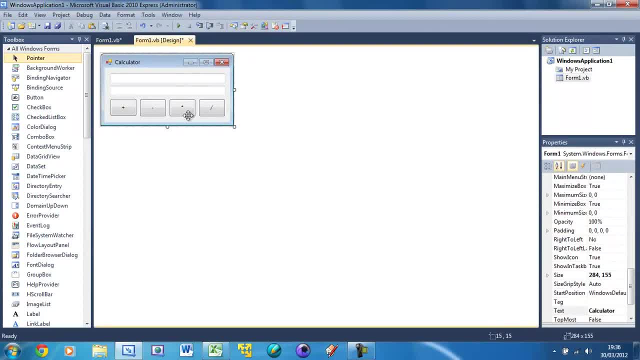 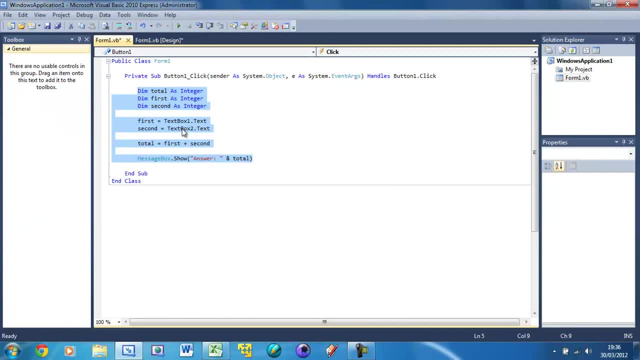 Like that And the times one. You can't really make it out clearly, But that is an asterisk, So shift and eight. So if we go back to our code now And we copy all this code that we just typed out, 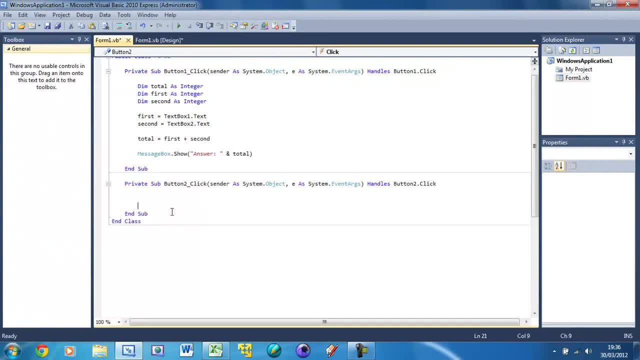 Close that And go to minus And we can just paste it in here And since this is the operator, we can change it. So I'm going to change that to minus. So it's going to be first. So the first variable, minus second variable. 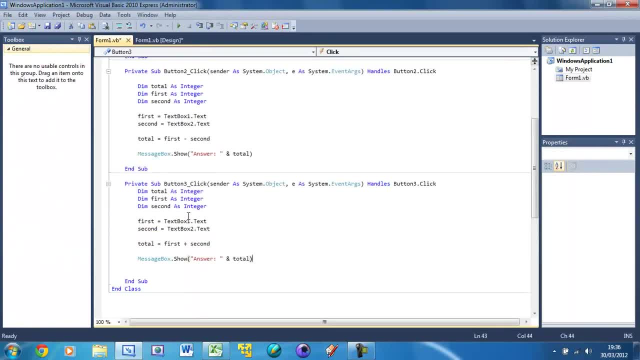 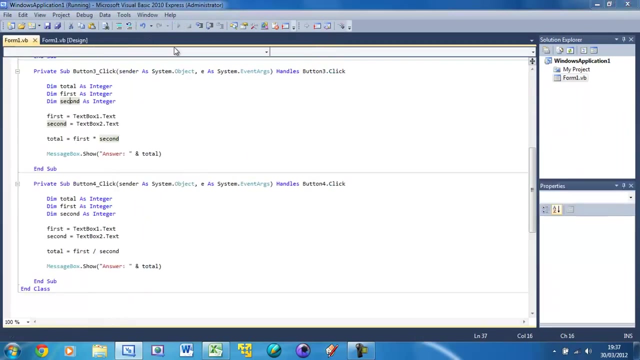 And go into the times. one: Paste that, Paste that in again, Neaten it up a bit And put times there. So again, that's an asterisk Divide. Paste that in And do forward slash. So now, if we run this,